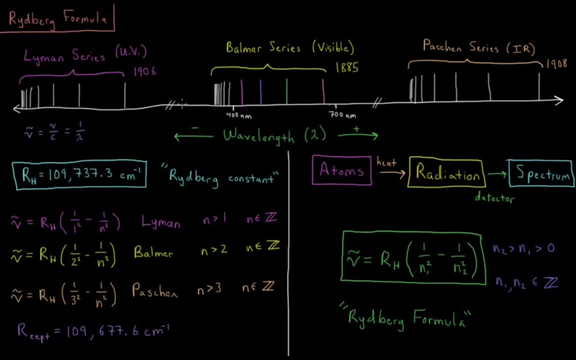 a specific value. So then later on, in 1906, Lyman discovered in the ultraviolet range another set of these kind of quantized wavelengths on the spectrum. He discovered that the same thing as Balmer, but in the UV, That there was one peak and then another one, and then. 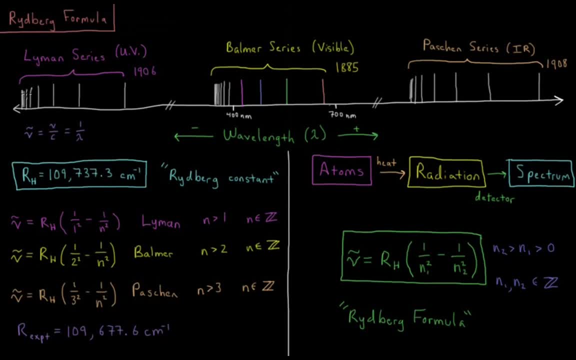 a third. that got closer and then closer, and then closer until they stopped at a specific value. And in 1908, Paschen discovered the same thing in the infrared region: That there was a specific peak, then another one, then they got closer and then they got closer. 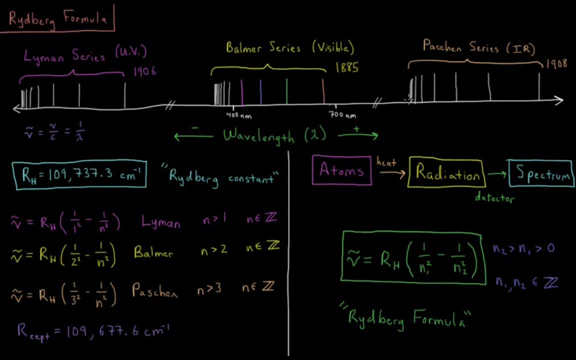 and closer, and closer, until a lot of them, and then they cut off at a specific value. So each of them thought: well, what can predict the location of these various lines here? So for Balmer, he found that if you do some constant times, 1 over 4, or 1 over 2, squared. 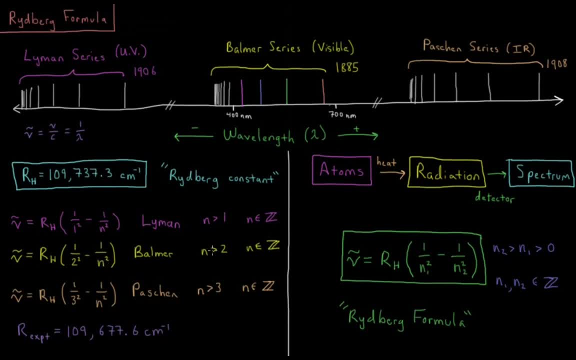 minus 1 over n, squared, where n is some number which is an integer greater than 2, so n can be 3,, 4,, 5,, 6,, 7,, 8,, 9,, 10,, 11,, 12,, 12,, 13,, 14,, 14,, 15,, 16,, 17,, 18,, 19,, 20,, 21,, 22,, 23,, 23,. 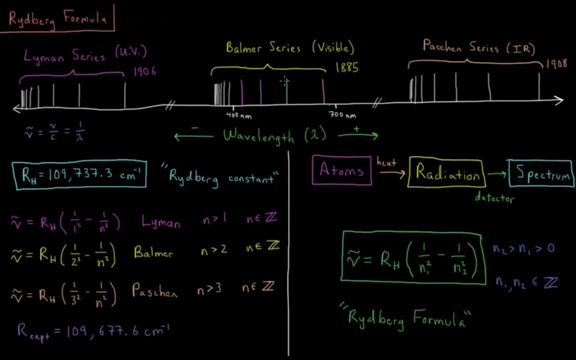 24,, 25,, 26,, etc. He discovered that these predict the locations of the lines in his series. The lines in the Balmer series are predicted by a constant times 1 over 2 squared minus 1 over n squared for n greater than 2.. 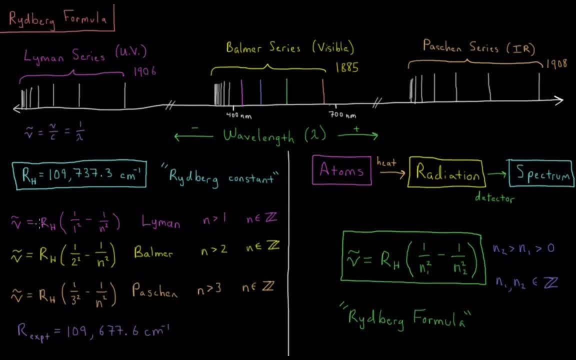 And then Lyman discovered a similar thing in the UV. It was a constant times 1 over 1 squared, minus 1 over n squared, but his n was any n greater than 1.. So 2,, 3,, 4,, 5,. 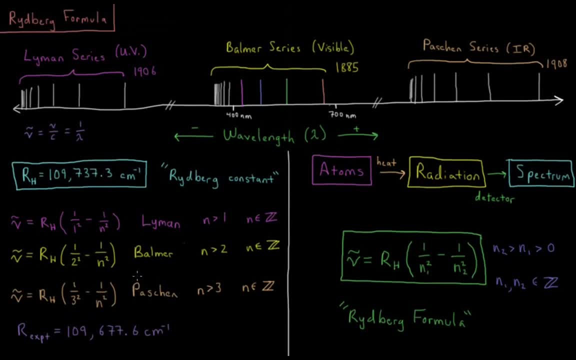 etc. And similarly for the passion series. you can fit a similar kind of formula: Constant times 1 over 3 squared minus 1 over n squared where n is greater than 3.. So this is: n equals 4,, 5,, 6,, 7,, etc. 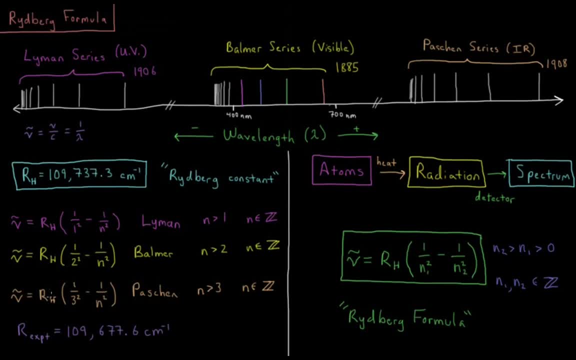 And the interesting thing is that all three of these fit to the same constant. Now, experimentally, this constant in wave numbers comes out to be 109,677.6 inverse centimeters. So that's equal to the frequency of the light divided by the speed of light. So this is also equal. 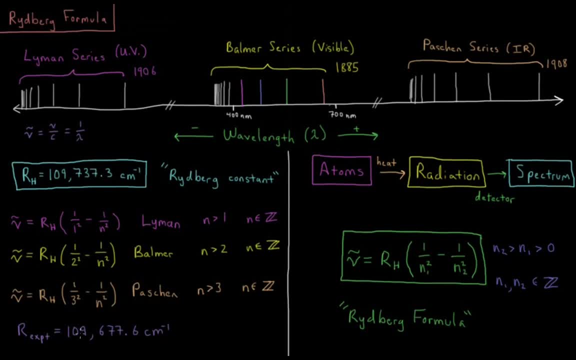 to 1 over the wavelength of the light. So this number, 109,677.6, falls in the UV range And this would be the number if you have the constant times. 1 over 1 squared, minus 1 over infinity squared, is this value? 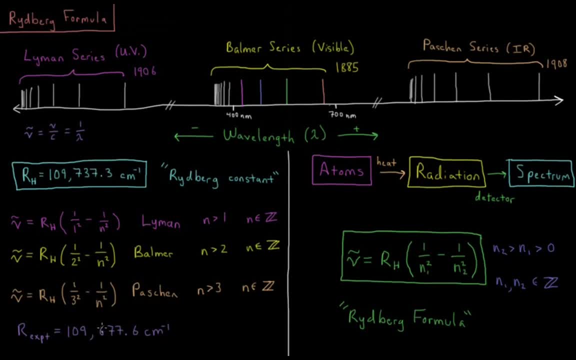 Okay, And this number is very, very close to a number which we know today as the Rydberg constant, named after Rydberg, who figured all this out. So the Rydberg constant which you'll find is 109,737.3 wave numbers, which is very close to this experimental number. 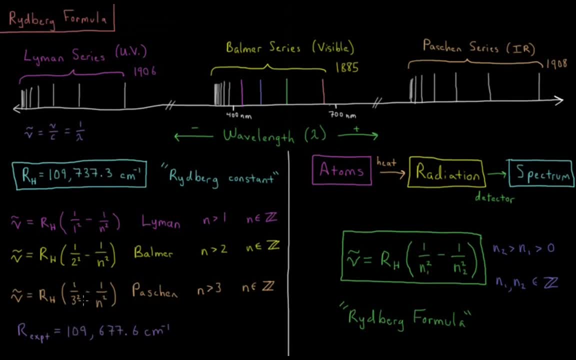 We'll talk about it in a few more videos, about what the difference between these two numbers and why it exists is Okay. So Rydberg discovered that not only is this true For these three series, but it's true in general of any series that follows the following: 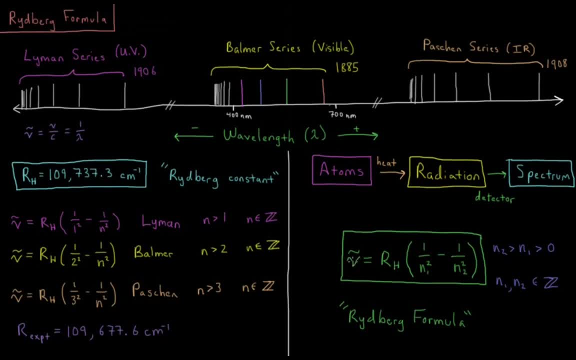 formula that the new bar, the inverse wavelength of the specific peak, is equal to this Rydberg constant times, one over N squared, minus one over N2 squared. So N2 has to be a number which is bigger than N1, which has to be a number which is bigger. 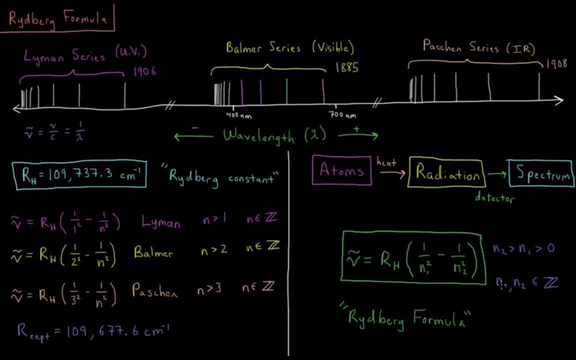 than zero and they are both integers, So they can both have values of one, two, three et cetera, And N2 has to be bigger than N1. And this formula overall is called the Rydberg formula and it predicts any possible peak. 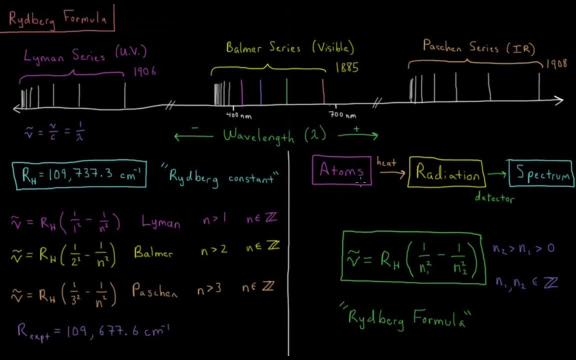 on a spectrum of hydrogen atoms. So any wavelength of radiation that a hydrogen atom is going to emit is going to be predicted by this formula. So this is kind of interesting that there are two integers in there for what radiation a hydrogen atom can emit.